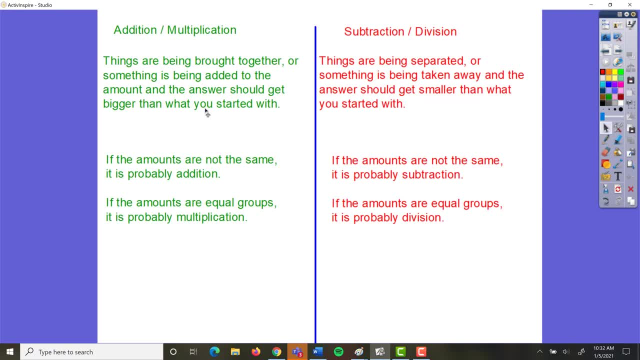 If something is being added to something else, or if different things are all being brought together into one big group, then that is going to be either addition or multiplication. Now, the way you can tell which one it's going to be: if things are being brought together that are equal amounts, that's going to be multiplication. 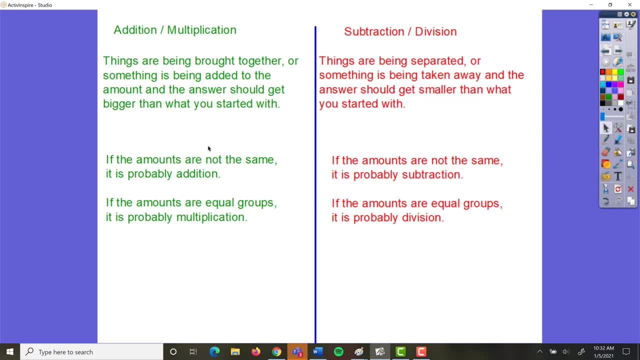 If things are being brought together that are unequal amounts or that are not the same amount, then that's probably going to be addition In subtraction. on the other hand, things are being taken apart, They're being separated, Or one thing is being taken away from another. 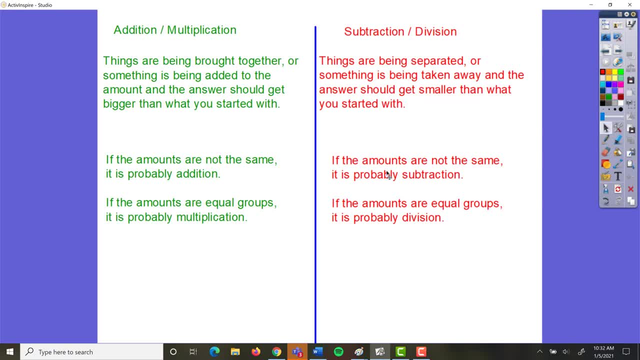 Again, you can tell whether it's going to be subtraction or division, because if the amounts are different, it's going to be subtraction. If it's equal groups of the same amount, then it's going to be division. So let's take a look at this in some actual problems. 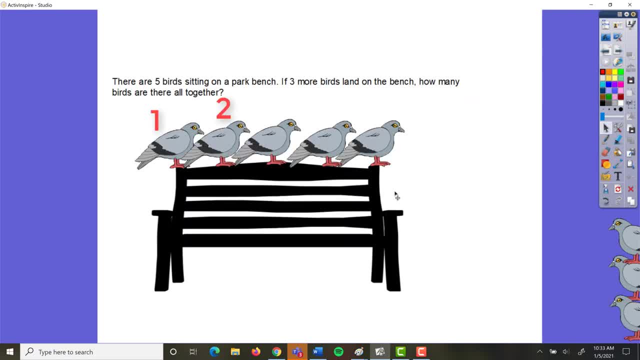 So let's say we have a problem that says there are five birds sitting on a park bench. If three more birds land on the bench, how many birds are there all together? So we're starting out with five birds and then three birds are being brought into the group. 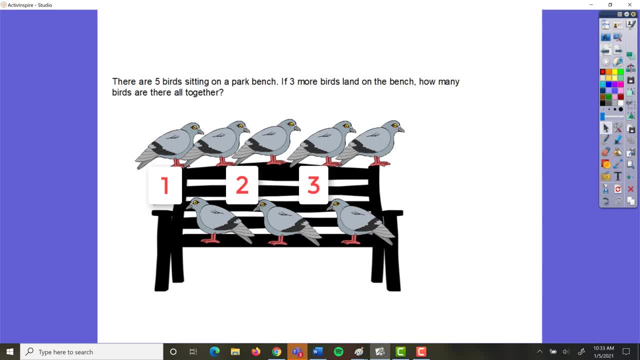 So we are bringing things together. So this is going to be either addition or multiplication. Now, were the two amounts that were being brought together the same or were they different? It was five birds And then we brought in three birds, So the numbers being brought together are different. 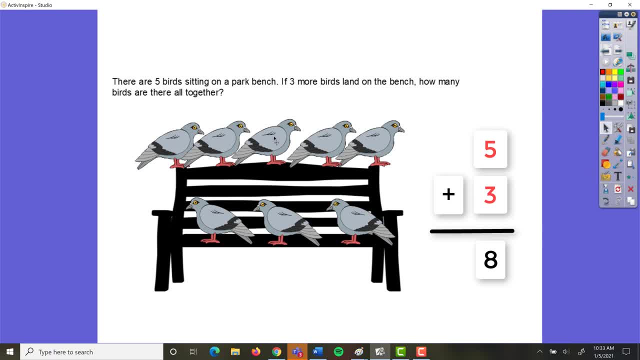 So this is going to be addition. Five plus three equals eight. So let's take a look at if this were a subtraction problem. So there are eight birds sitting on the bench and three of the birds fly away. So one amount is being taken away from or split apart from the other. 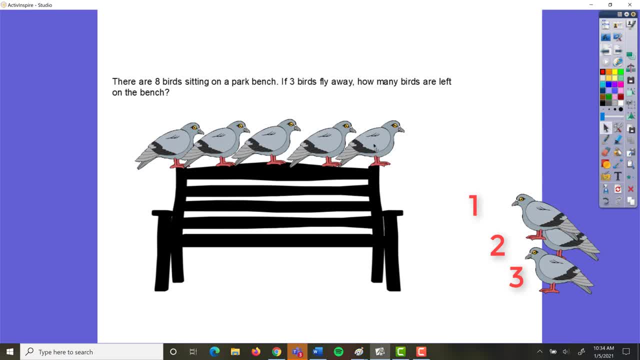 So that's subtraction. The other is being taken away from or removed from the other, And we're going to wind up with an answer that's smaller than what we started with, Because we started with eight and we know that three are being taken away from that amount. 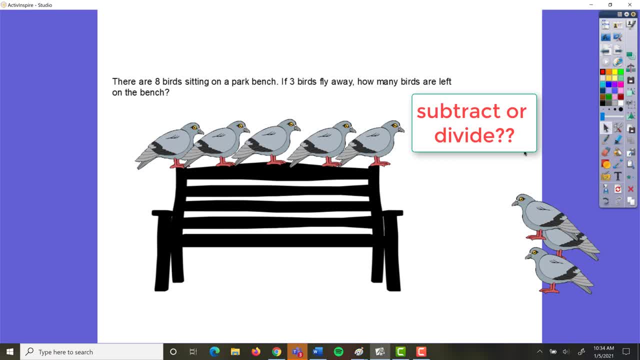 Now that's going to be subtraction or division, because things are being split apart or taken away or removed. The number is going to get smaller. So is it subtraction or division? Well, were the amounts equal or were they unequal? Eight birds and we took away three. 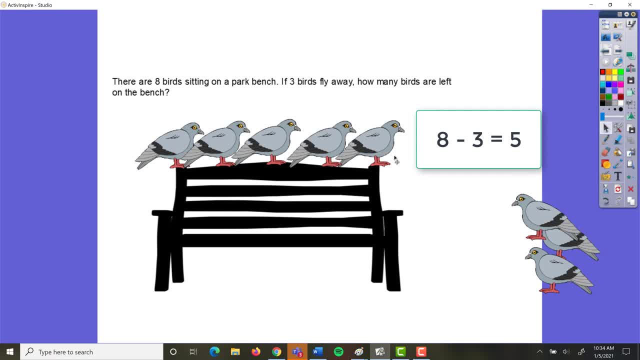 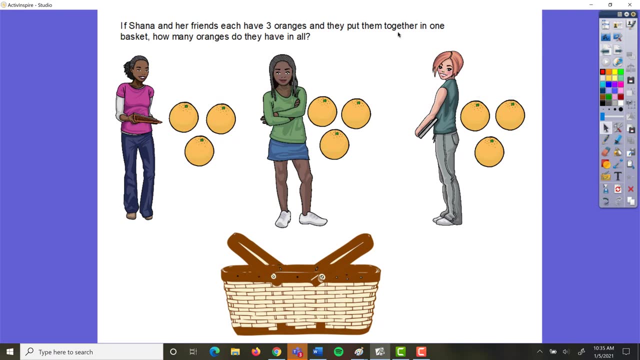 So no, those are not equal amounts, So this is subtraction. So we have eight birds minus three birds, We're left with five birds. Okay, let's take a look at some additional problems. If Shanna and her friends each have three oranges and they put them together in one basket, 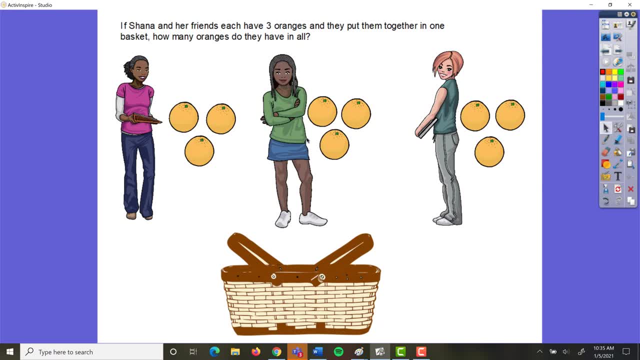 how many oranges do they have in all? Well, are their oranges being split apart or are they being put together? In this case, they are putting them all together into a basket. So her three are going to go in the basket. Her three are going to go in the basket. 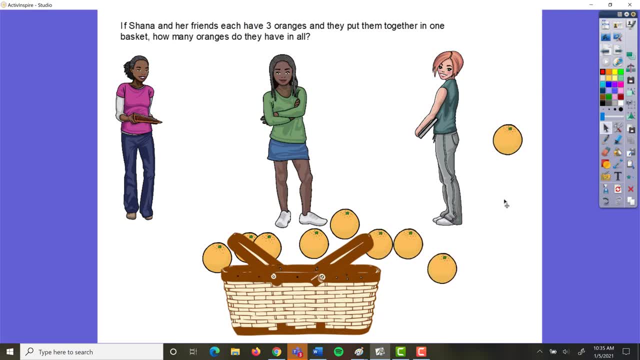 Her three are going to go in the basket. So we're taking these amounts and we're putting them together. So this is either addition or multiplication. Now were the amounts the same or were they different? Each girl had three, So this was a group of three. 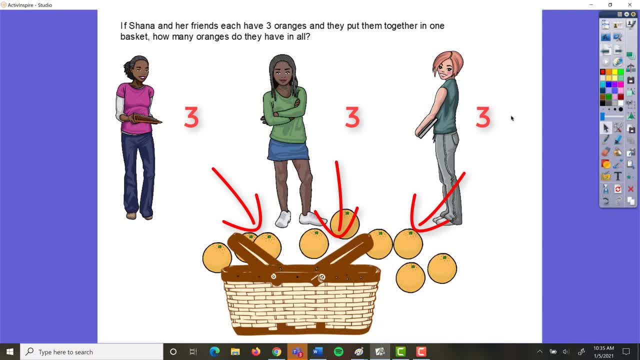 This was a group of three And this was a group of three. They are equal amounts being brought together. So this is multiplication And it is going to be three oranges times three girls, for a total of nine oranges. Okay, let's look at it going the other way. 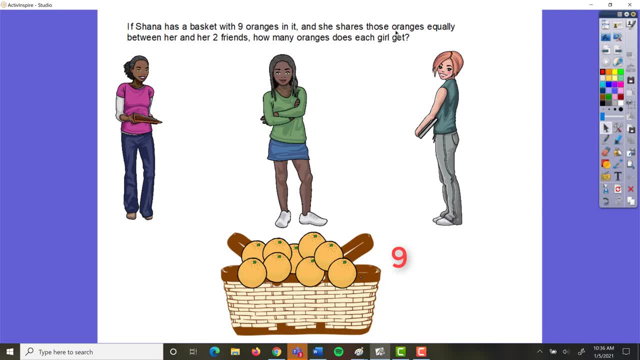 If Shanna has a basket with nine oranges in it and she shares those oranges equally between her and her two friends, how many oranges does each girl get? Are these oranges being taken apart or are they being put together? They're being taken apart. 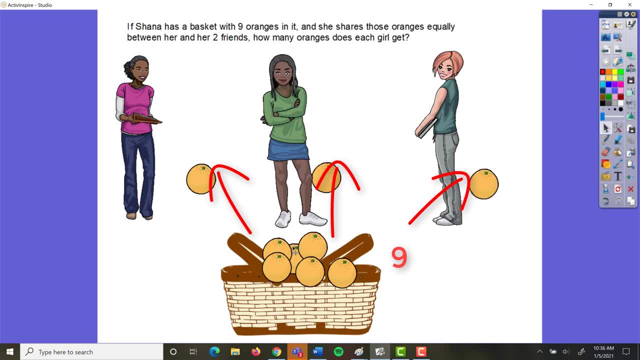 Each girl is getting some oranges right Now. are they going to get equal amounts? So that's going to be subtraction or division. because each girl is getting oranges, They're being separated- Subtraction or division. Well, are the amounts equal? 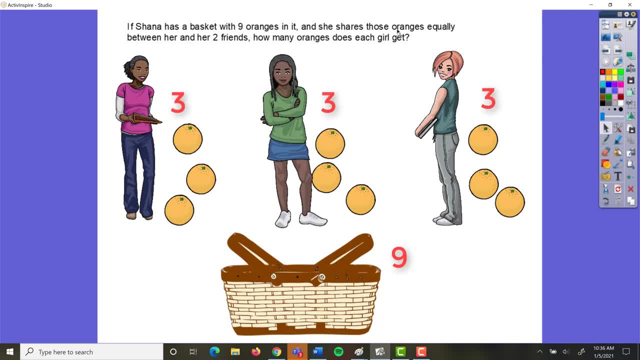 or are they each going to get a different amount? Well, it says that they need to share them equally, So each girl is going to get the same number. That means it must be division, because we're talking about equal groups. That's really pretty much how you decide. 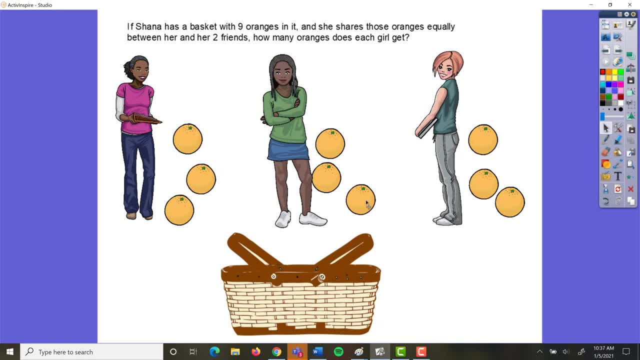 Now, some problems are more complicated than that and some problems are a little bit harder to understand- whether things are being taken apart and put together and whether the amounts are equal or not- But as a general rule, that's a good guide, So let's review. 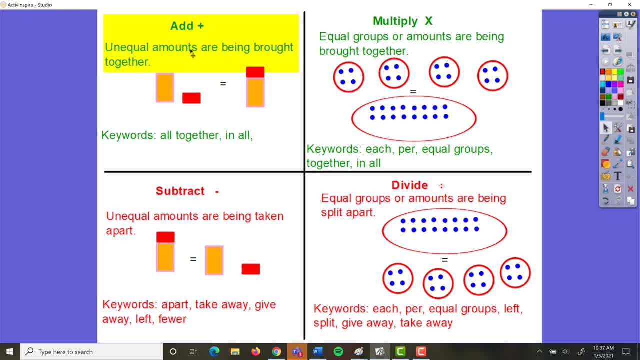 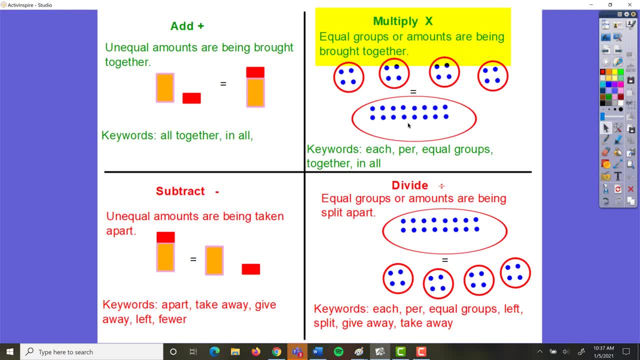 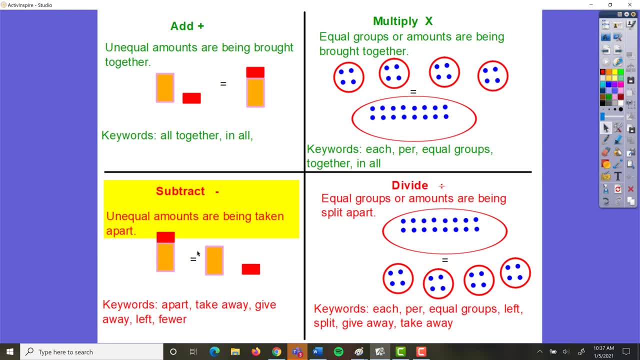 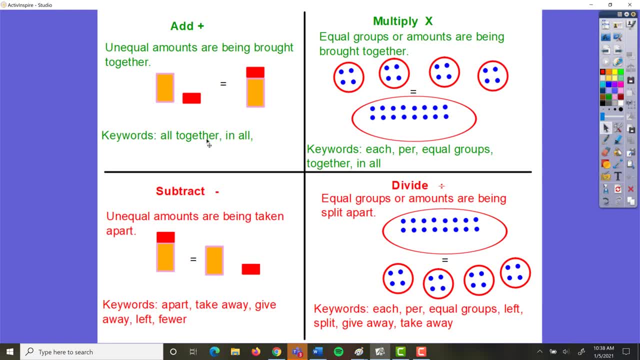 These aren't 100%. Sometimes, again, word problems can be worded in a way that's a little bit confusing, But as a rule any word that tells you things are being brought together, all together, in all, they put them together whatever. 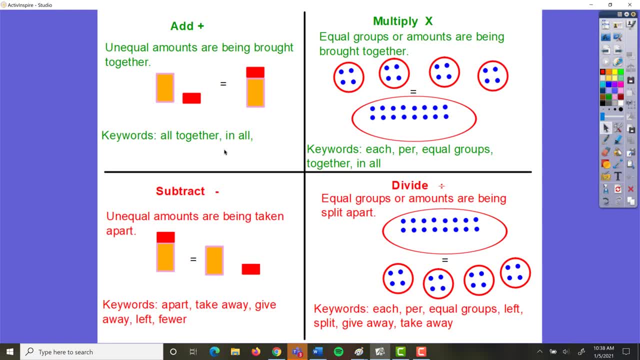 things that tell you things are being one thing is being added to another. words that tell you things are being brought together will indicate it's going to be addition or multiplication, So you'll see the same words in both, But the difference is. 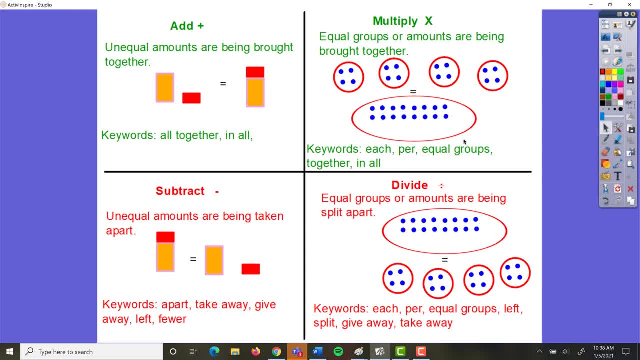 if you see each, per or equal groups, you know it's probably going to be multiplication. Same thing with subtraction: Any word that tells you things are being taken apart, that you're going to have fewer left behind. there's going to be something left.